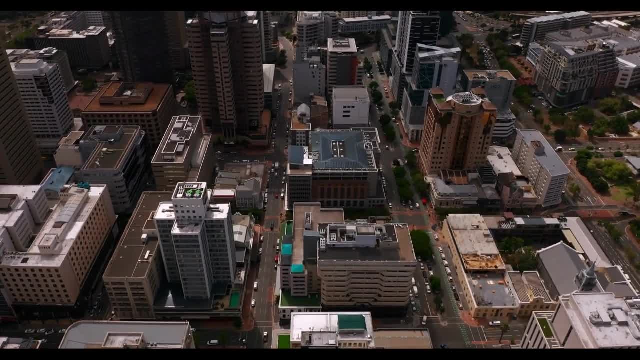 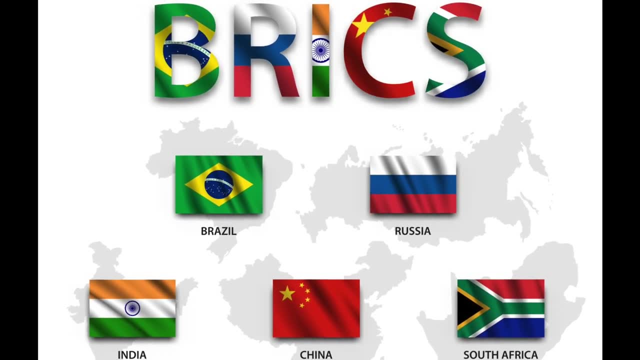 It was promoted as the economic star of the continent. It even hosted the 2010 World Cup and is part of the BRICS, along with Brazil, Russia, India and China, a group of economies that enjoyed rapid economic growth and will supposedly dominate the world economy by 2050. 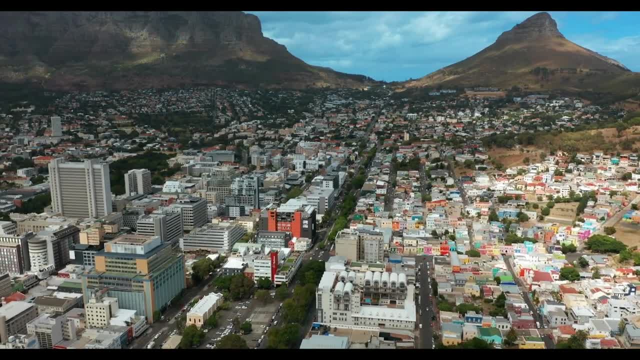 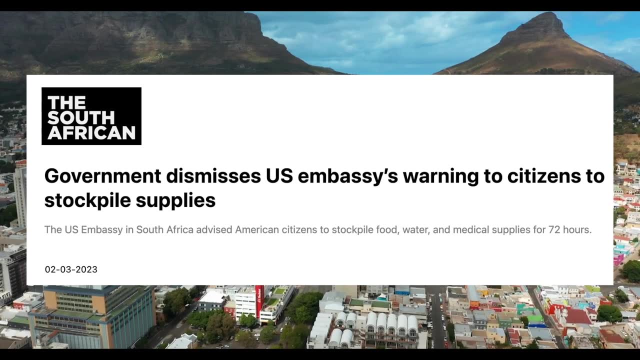 However, in early 2023, the US Embassy in Pretoria, the capital of South Africa, advised Americans living in this country to have at least 72 hours of food, water, medicine and hygiene items in case of a possible total collapse of the South African power grid. 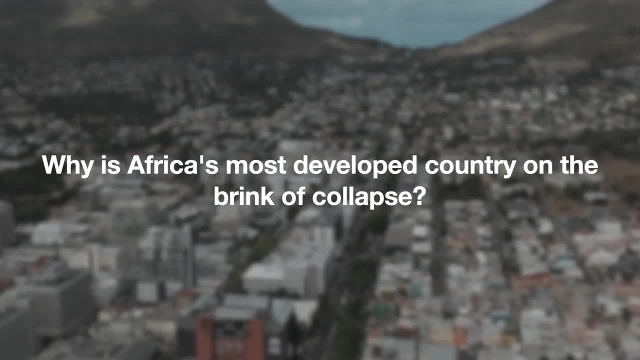 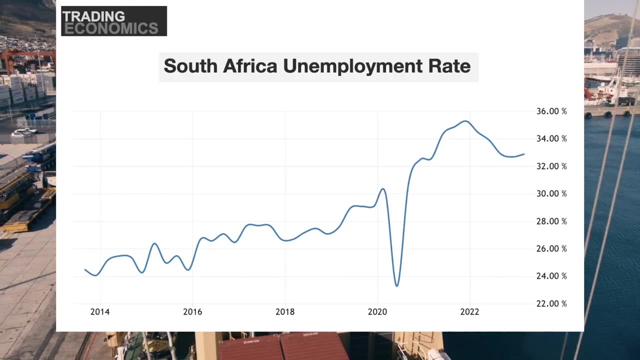 So the question is: why is Africa's most developed country on the brink of collapse? A few statistics could sum up the current state of the South African economy. It has an unemployment rate of 33%, one of the highest in the world- And youth unemployment. 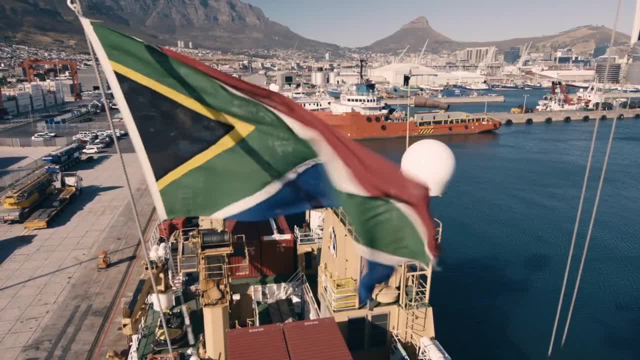 between the ages of 15 and 24 is 62% By 2021,. the percentage of the population living in poverty was 6%. The US Embassy in Pretoria, the capital of South Africa, has a population of 6%. The 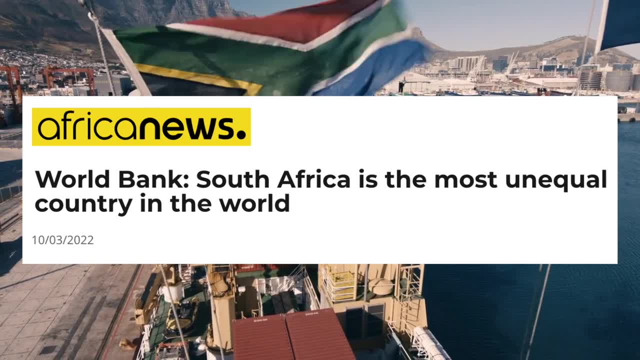 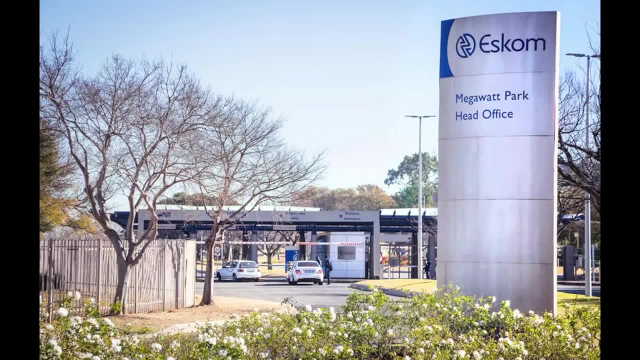 US Embassy in Pretoria is 63%. It is said to be the most unequal country in the world and occupies the first places in the ranking of crime rates. But that's not all, because, in addition to South Africa's economic woes, there has recently been a crisis at Eskom, the state-owned company. 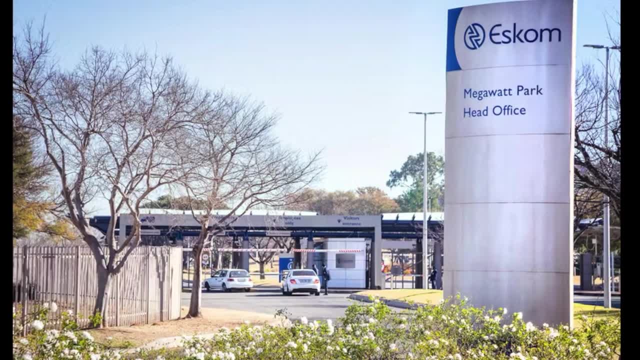 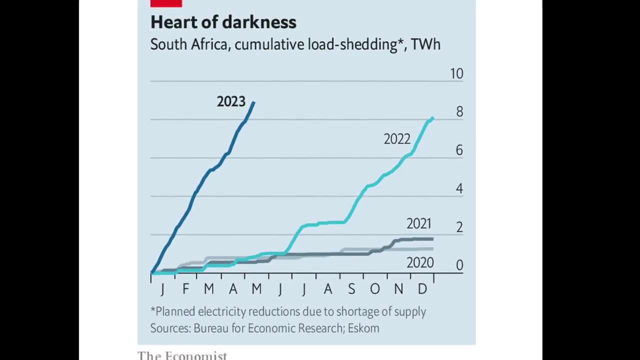 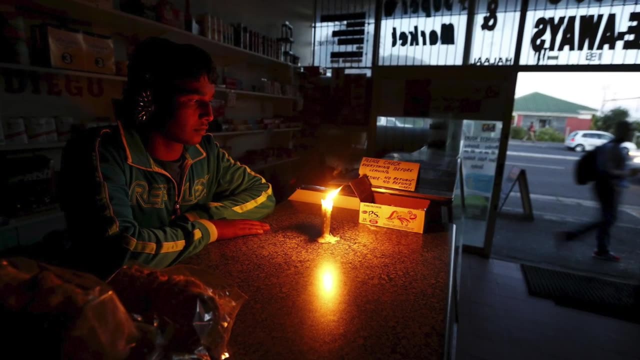 responsible for managing the country's electricity grid. In South Africa, blackouts doubled in 2022, and in 2023 they already reached a record high. There are days when the power goes out for 10-12 hours. First, blackouts were occasional once a month. Then they occurred two or three times a week. 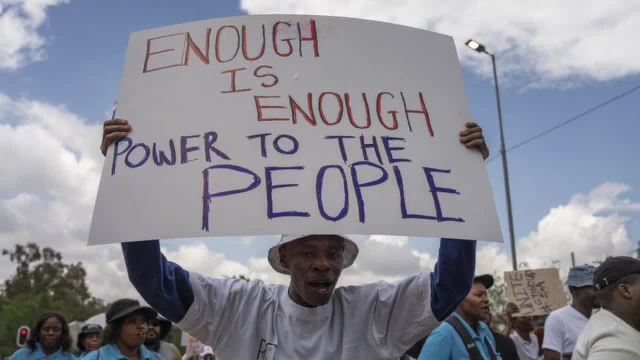 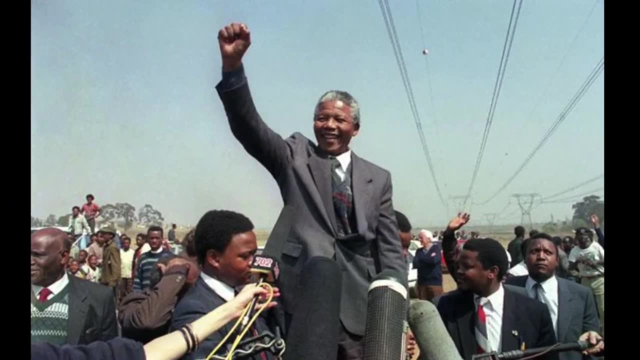 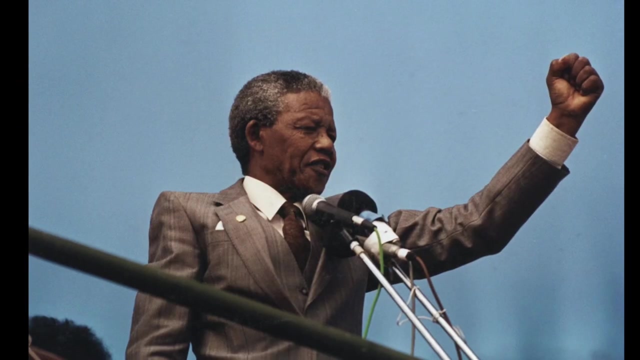 And now they are part of the daily routine. But how did one of the richest countries in Africa come to this situation? It turns out that when Nelson Mandela became president of South Africa in 1994, cheap electricity was seen as a benefit of freedom, so price hikes were avoided at all. 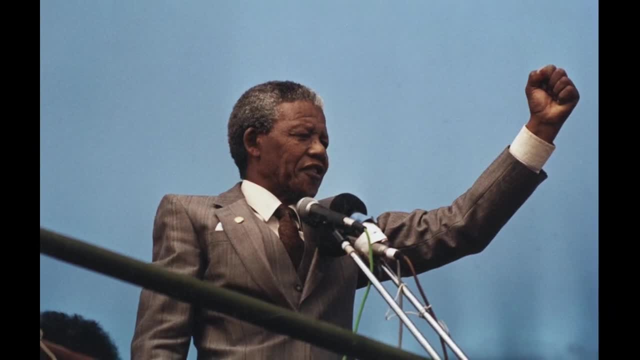 costs for fear of public backlash. So the lack of investment at the expense of offering cheap electricity should not be a problem. The US Embassy in Pretoria, the capital of South Africa, is the only country in the world that has ever invested in a huge amount of electricity. The US Embassy in Pretoria, the capital of South Africa, has been a great source of electricity, But the electricity crisis has largely been a result of the lack of investment in electricity. There is a great deal of demand for electricity, But the problem is that many South Africans simply refuse to pay their electricity bills And likewise it would be very unpopular to cut off service to so many people. For example, in the city of Soweto, with more than 1 million inhabitants, an estimated 80% do not pay their. 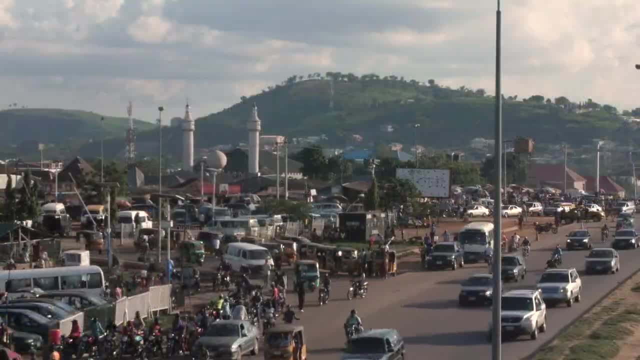 bill. But even if they were to cut off the electricity supply to defaulters, illegal service connections would make this problem much more serious. And the problem is that many South Africans simply refuse to pay their electricity bills and likewise it would be very unpopular to cut off service to so many people. 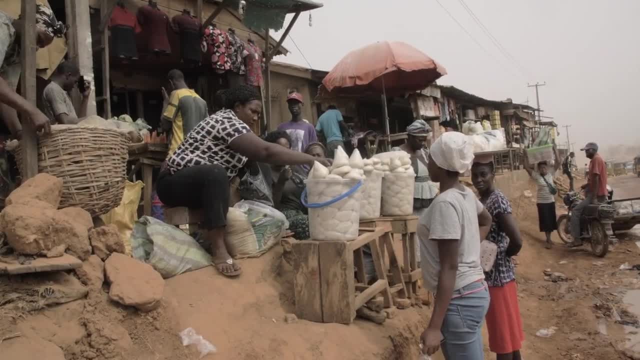 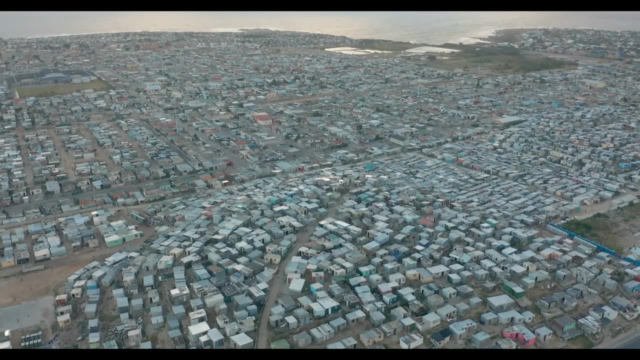 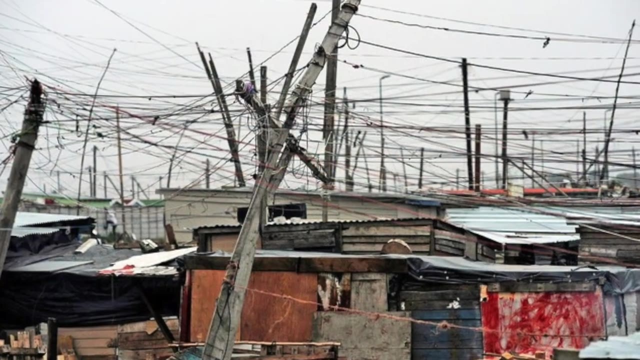 bills And likewise it would be very unpopular to cut off service to so many people. For example, in the city of Soweto, with more than one million inhabitants, an estimated 80% do not pay their bill. But even if they were to cut off the electricity supply to defaulters, illegal service connections. 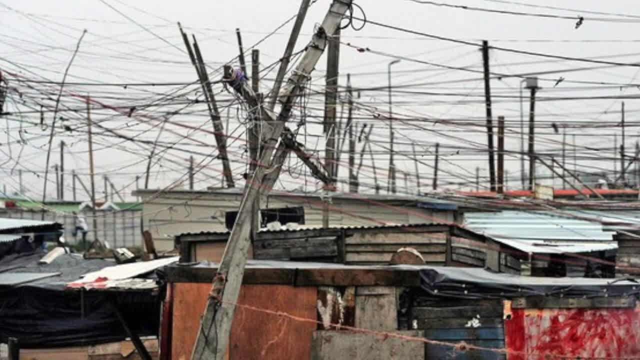 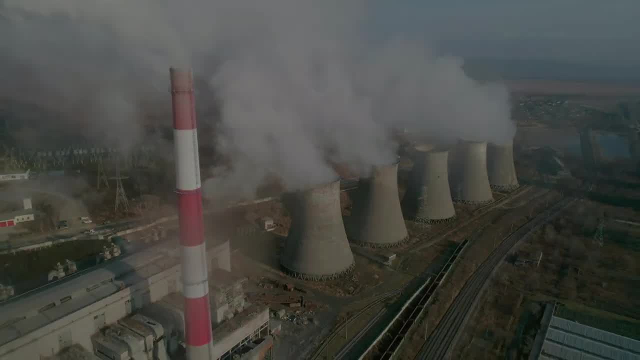 would make this measure useless. On the other hand, for decades the state-owned company has been plagued by corruption and mismanagement. Some blame the looting of the company on the Gupta brothers, Three men from India who came to South Africa in the 1990s and with the help of former 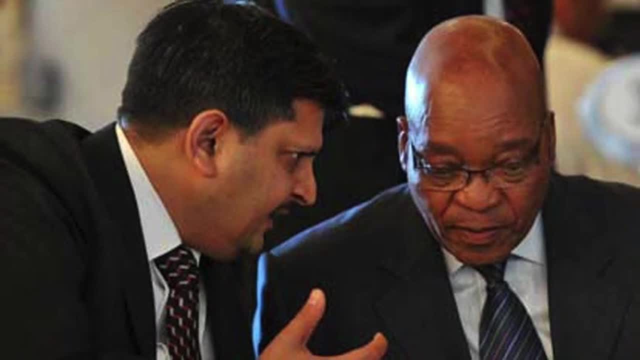 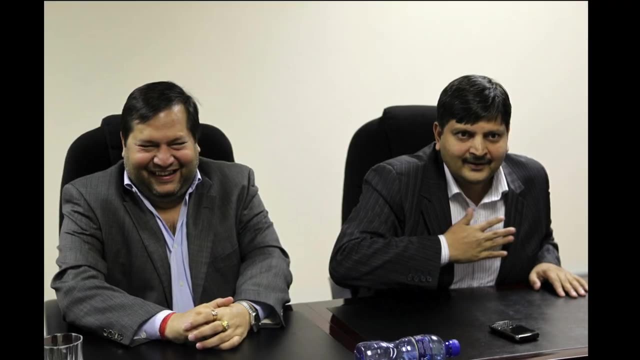 South African president Jacob Zuma left the company with $23 billion worth of debts. In 2018, they fled to Dubai. Two of the brothers were arrested there, but were released after a court refused to extradite them for trial in South Africa. 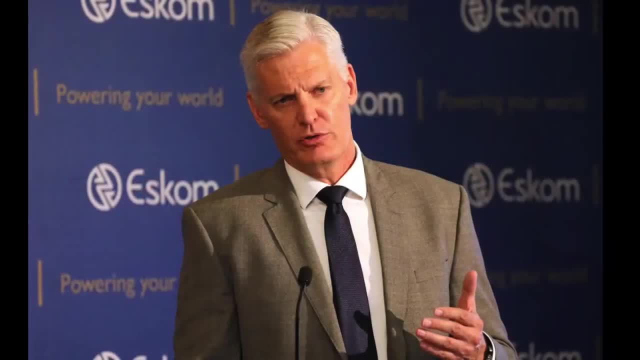 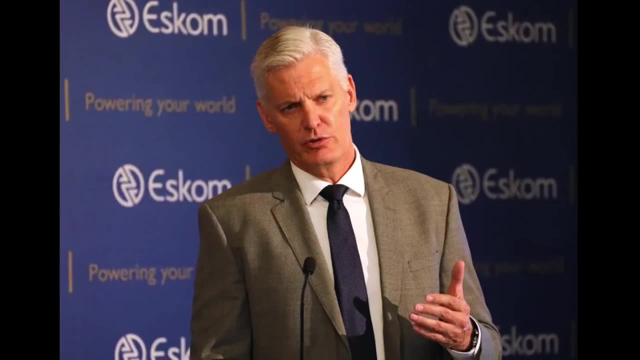 After the Gupta brothers fled, Andrew de Rutter took over the management of the company and tried to end the company. Andrew de Rutter tried to stop corruption but was unable to do so because, according to him, the national government intervened to sabotage his anti-corruption efforts. 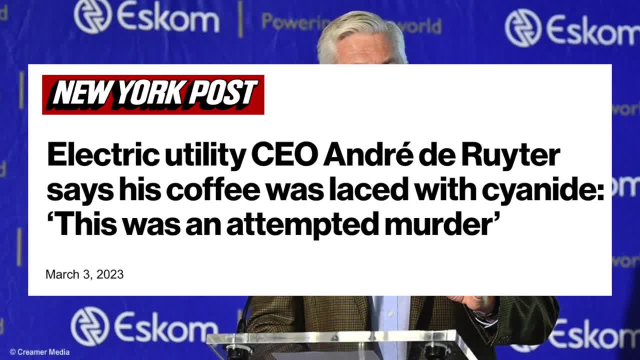 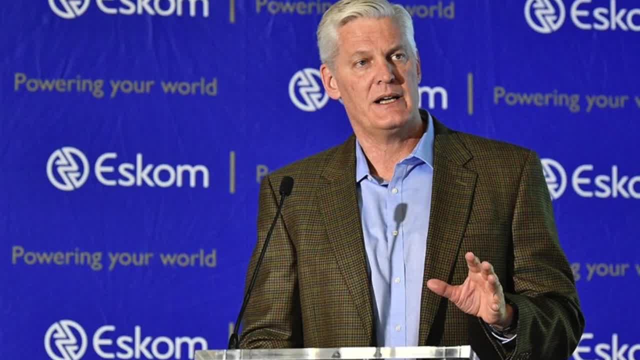 In fact, an attempt was made to assassinate Andrew de Rutter by putting cyanide in his coffee, and months later he resigned from his job, From which it can be deduced that he did have enemies who opposed his attempts to eliminate corruption and blackouts. 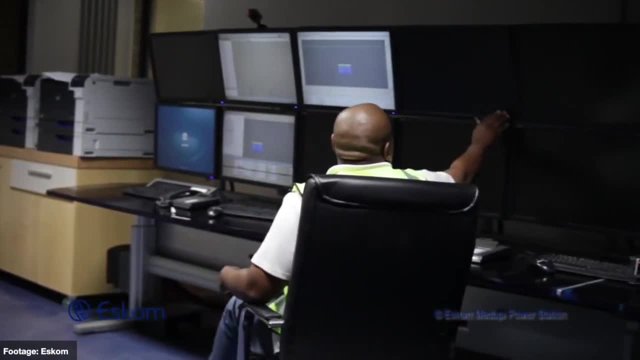 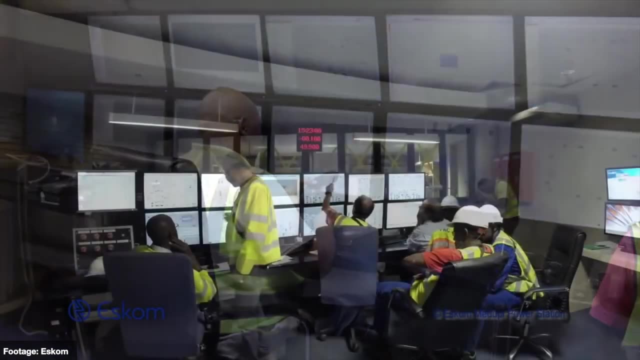 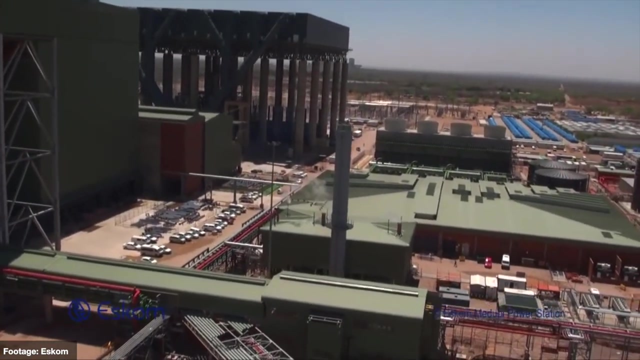 Another factor exacerbating the electric company's crisis is that it is constantly under attack by local criminal cartels. It is common for contractors to purposely damage the infrastructure of power plant so that corrupt repair companies can fix the damage at an inflated cost. Another tactic used by criminals is that, since more than 80% of South Africa's electricity 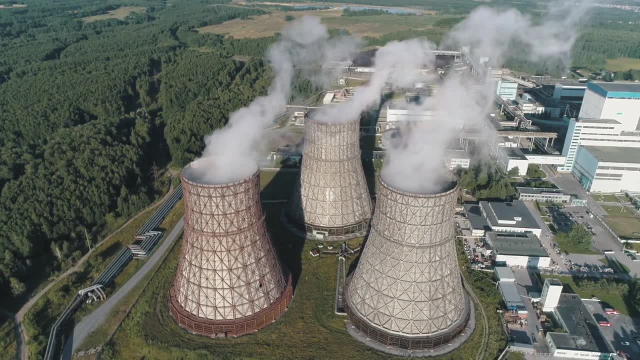 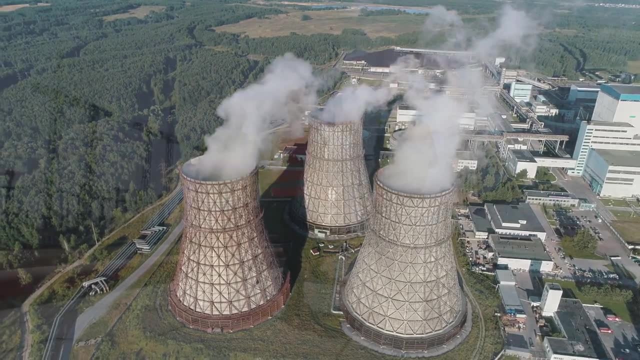 is generated by coal-fired power plants. criminals often steal good quality coal from the company and exchange it for poor quality coal. Such sabotage is a daily affair. A South African journalist, Kyle Cowan, investigated several failures at Eskom's facilities, such 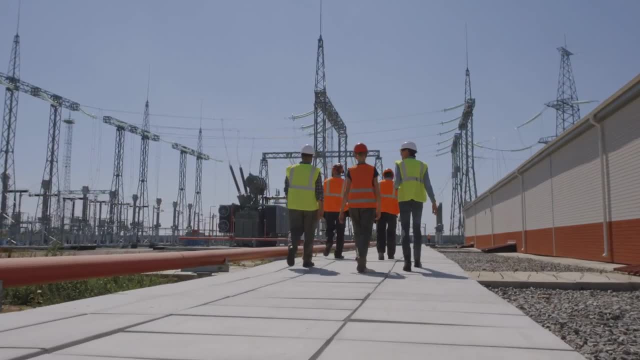 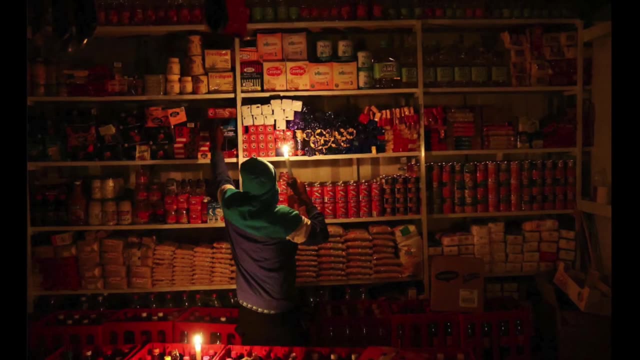 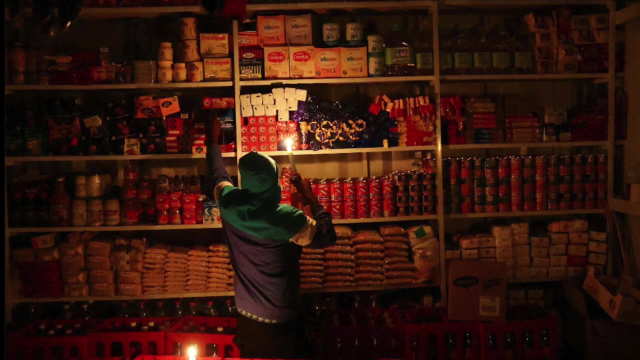 as downed power pylons, jammed coal mills and discovered many cases where sabotage was the most likely cause. This is how Eskom has been forced to impose blackouts for the sake of electrical reasoning, And this generates serious economic, humanitarian and health consequences. 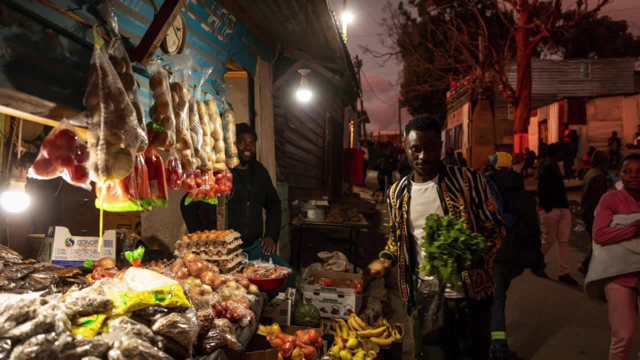 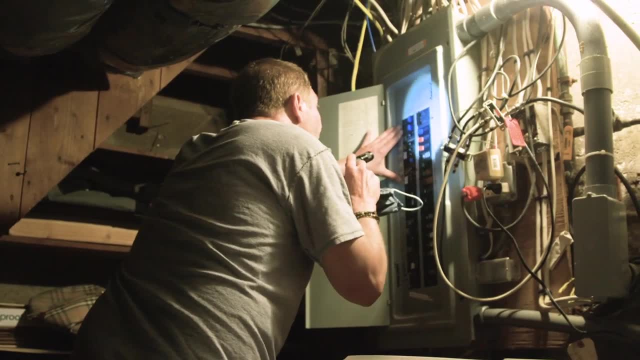 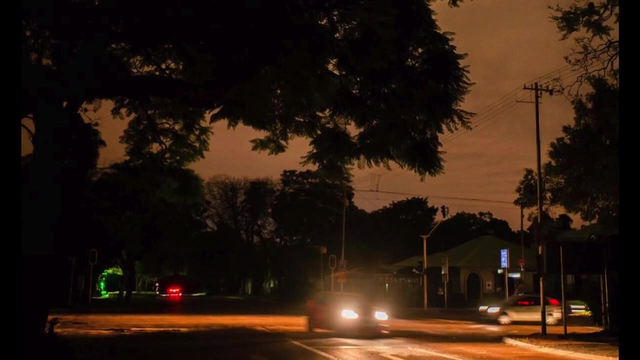 Blackouts which occur throughout South Africa affect homes, businesses, street lighting, traffic lights and hotels. Power outages can also affect water availability, internet connectivity and cell phone network coverage. Power outages can increase crime. For example, when traffic lights stop working, traffic jams occur, which criminals take advantage. 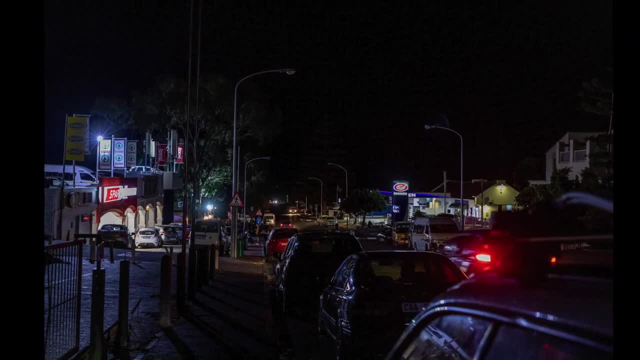 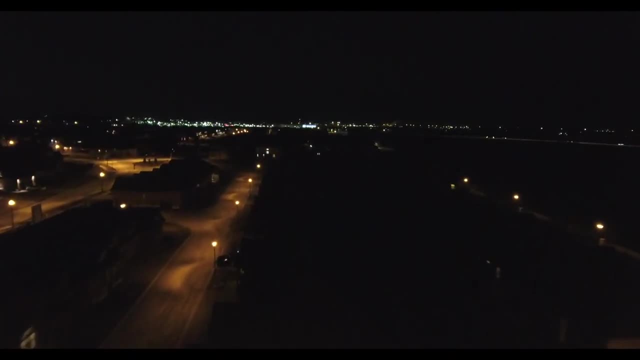 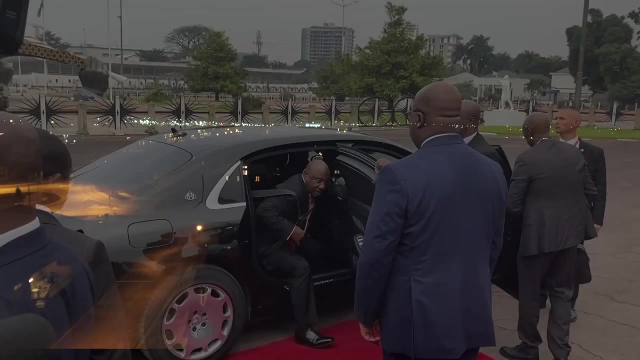 of to commit crimes against drivers. In addition, residences can be targeted when the lights are off. street lighting does not work and security systems stop responding. In total, these outages are estimated to have cost the South African economy $50 million per day. 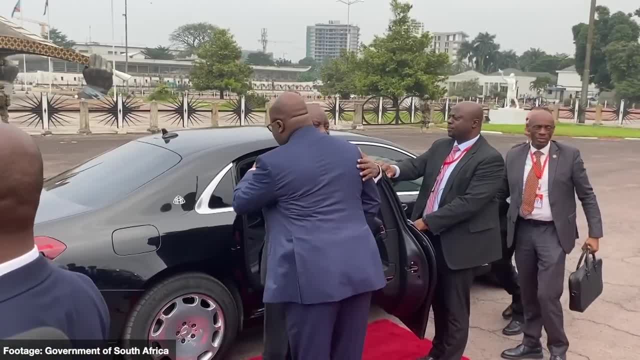 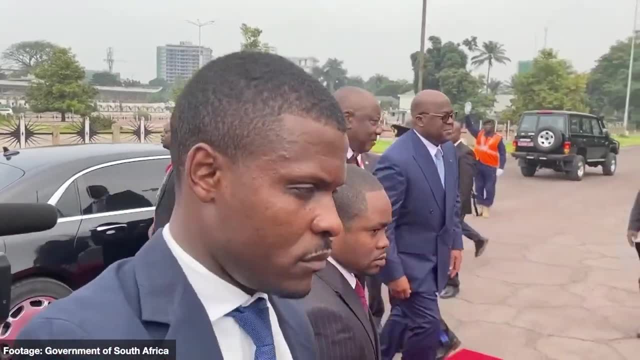 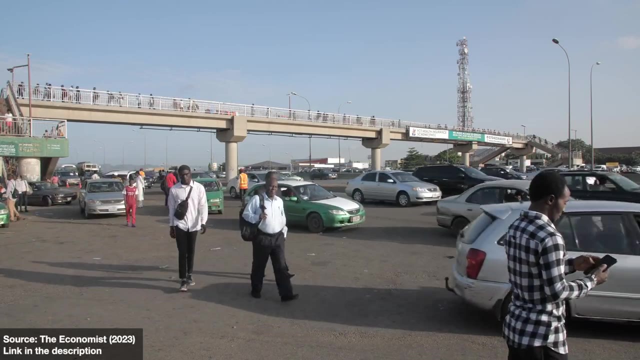 Government incompetence, corruption and crime have left critical infrastructure in Africa's most industrialized nation in ruins, forcing companies to step in to fix the problems and replace the state. For several years now, companies have been sending staff to help run government departments by paying their salaries. 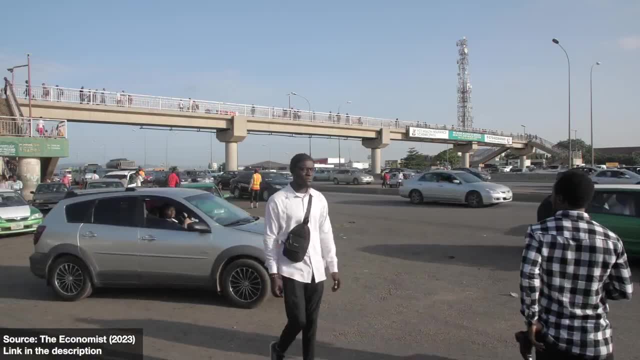 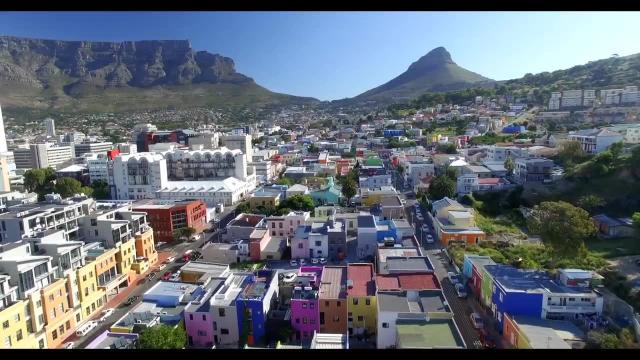 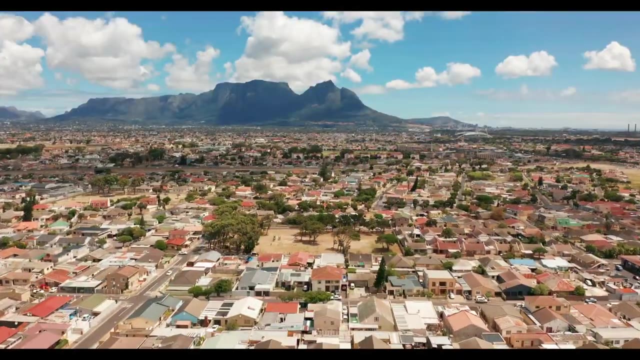 Corporate lawyers work in the public prosecutor's department and bankers in the Department of Industry. With their staff, the companies repair potholes in the roads, pay for some fire vehicles and make sure that some areas are well-lighted. The fact that private companies are replacing the state in its basic functions was unthinkable. 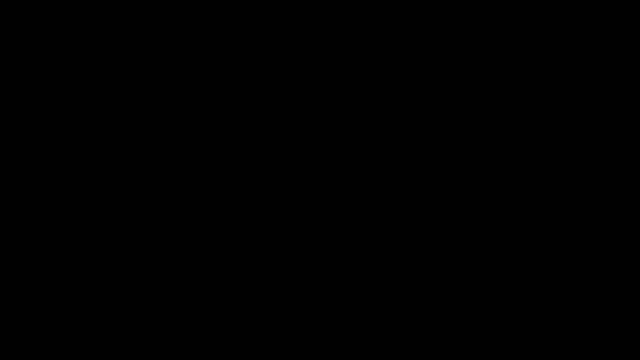 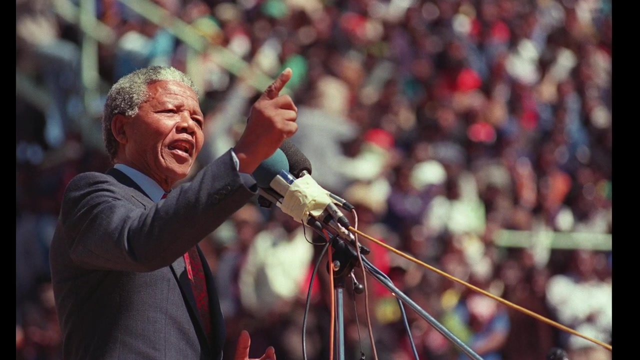 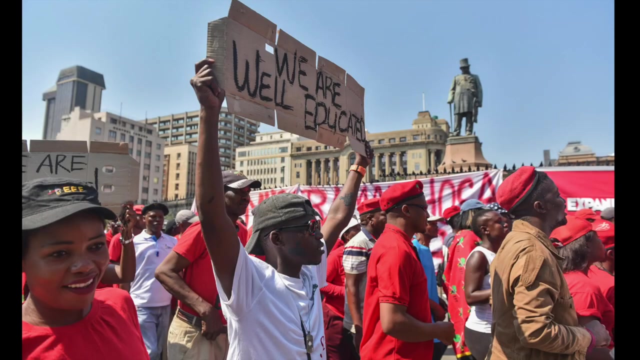 a few years ago. The African National Congress, Nelson Mandela's party, has ruled the country since 1994.. They promised an efficient, state-run economy that would uplift the oppressed black majority, But decades later, the government's role as a provider of basic services is virtually